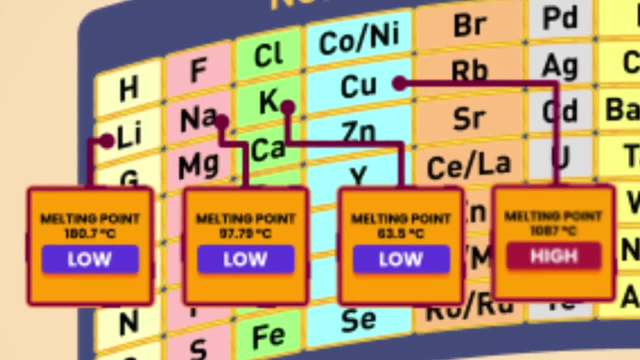 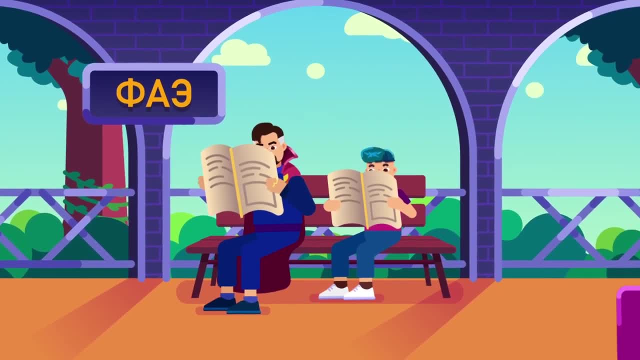 down and made some elements being grouped together despite not having similar properties. Then came Dimitri Mendelsohn Mendelsohn, a Russian chemist, who looked at the periodic table that was being used at this time. He noticed a few problems in it. Some elements were being put into groups with other elements. 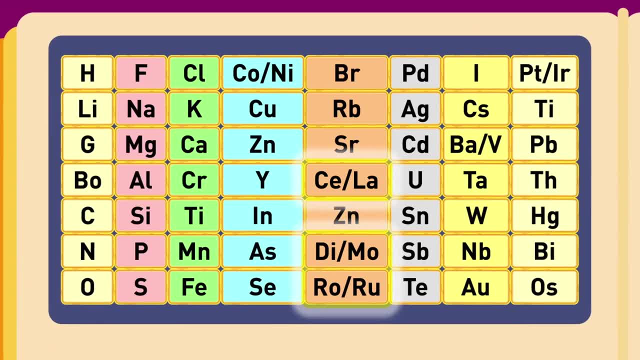 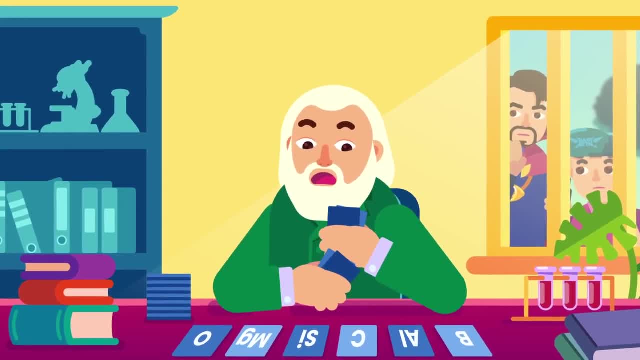 which they did not react similarly to, and some boxes of the periodic table were even having multiple elements put into it. Mendelsohn started writing each known elements on cards and kept rearranging them like playing cards. After relentless work, he fell asleep and instead. 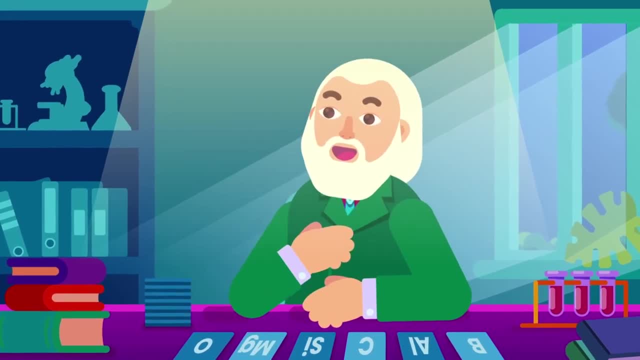 of getting nightmares. he got the idea about how his periodic table should be organized After a long period of thinking. he wanted to know if slash and divide would work. The only possible answer to this was the following: Mendelsohn found materials that were problematic. 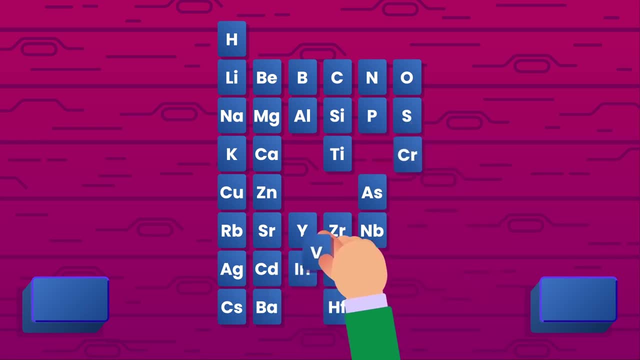 and placed them in groups that share similar properties, while making sure to keep one element in each box. This ended up leaving gaps in the periodic table that could be filled in with elements that were found later by other scientists. This was one of the main reasons his theory was. 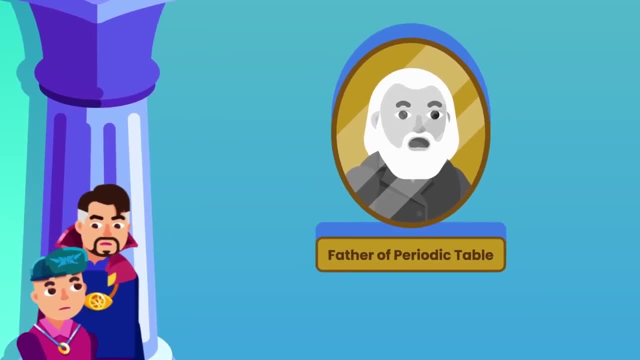 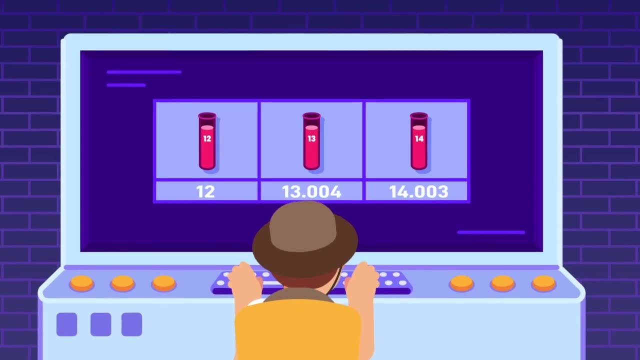 so readily accepted and in fact his design led him to obtain the nickname The Father of the Periodic Table. The other reason his theory was accepted was that the discovery of isotopes showed that we could not base the classification of the elements on the atomic 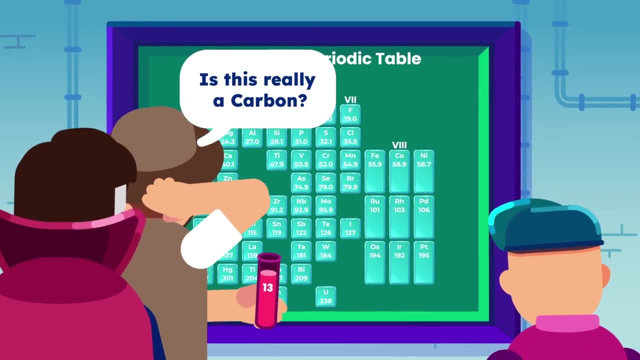 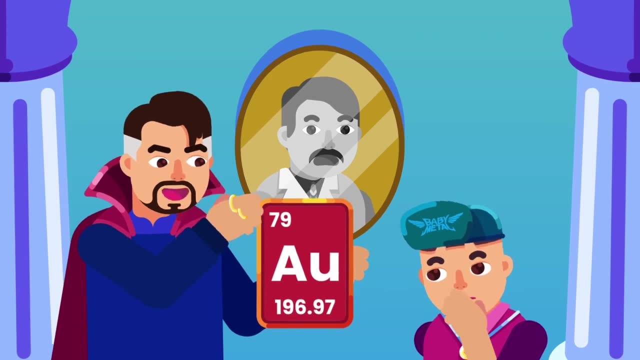 masses alone, like the previous scientists had done. This was improved better by young Henry Moseley, who deduced that the periodic table is best arranged based on its atomic number instead of its atomic weight. You can learn more about isotopes in our other video. 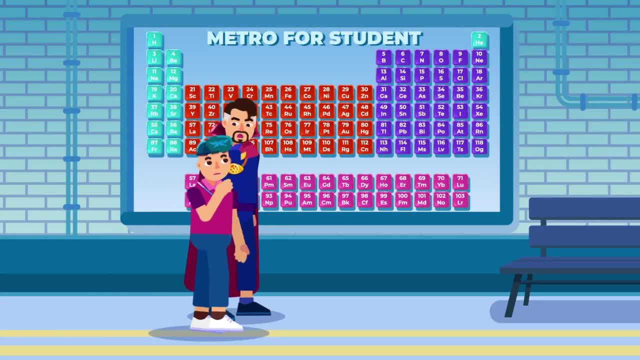 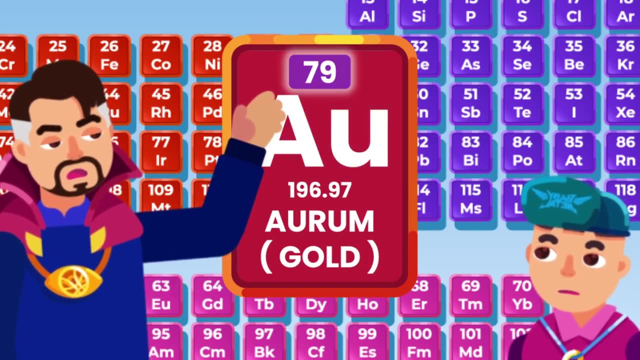 Today's periodic table of elements is an updated version of Mendeleev design. Each element is given a square in the table that tells us its name, its chemical symbol, its atomic number, the number of protons and its atomic mass- the number of protons and neutrons based on its isotope abundance. 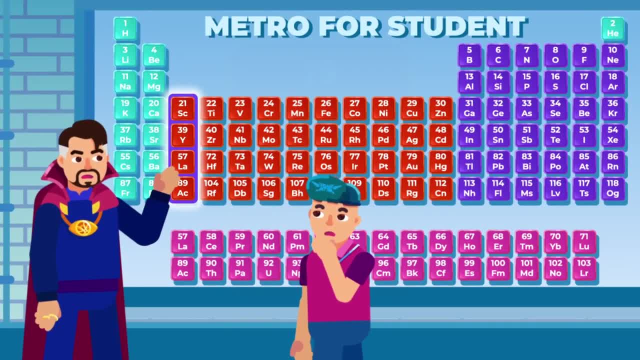 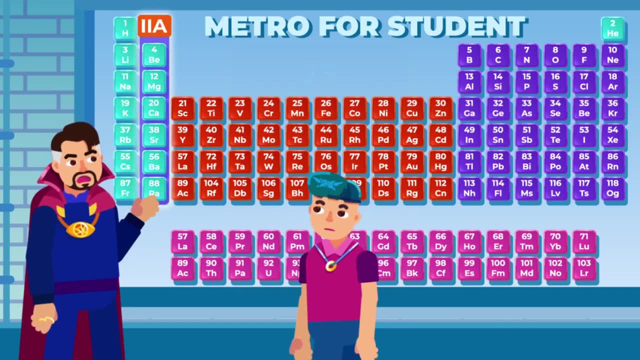 These elements are listed in order of increasing atomic number and are organized into groups, which are the vertical columns, and periods, which are the horizontal rows. Elements that were put into the same group were put there because they reacted similarly to other elements in that group And, although this wasn't known at the time, this was because